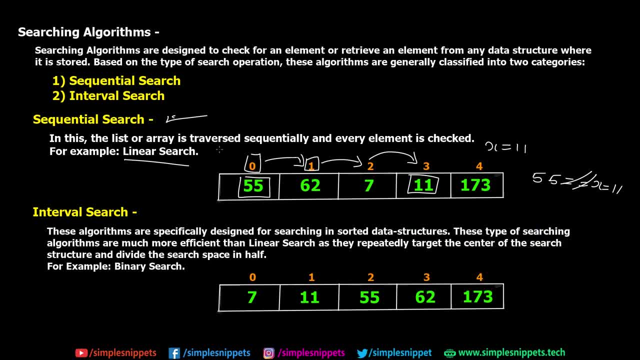 out. There are other topics in this playlist as well, And, with that being said, let's get started with today's topic, that is, Binary Search Algorithm. Now we'll divide this topic in two parts. In this part, we will discuss what exactly is the binary search algorithm. 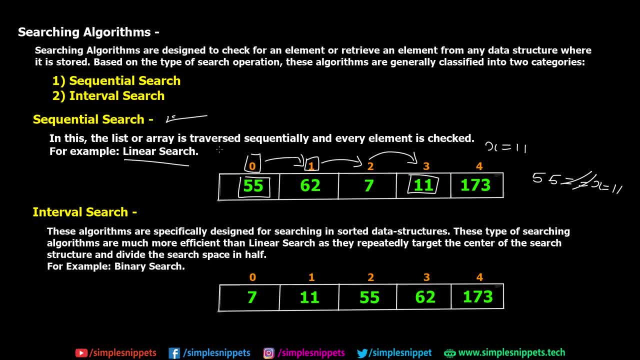 the working and the algorithm And we'll also take a diagrammatic representation and we'll take an example. And in part two- that is, in next video after this one, we'll actually implement the binary search algorithm using C++ programming And we'll convert the algorithm into actually the implementation part in a C++ code. Okay, 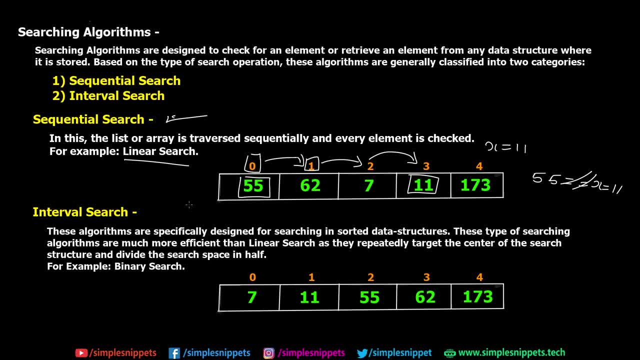 so let's get started Now. binary search algorithm is basically an interval search algorithm, So it is a type of interval search And it is not exactly a sequential search. So when I say it is not sequential search, binary search algorithm does not go from one index. 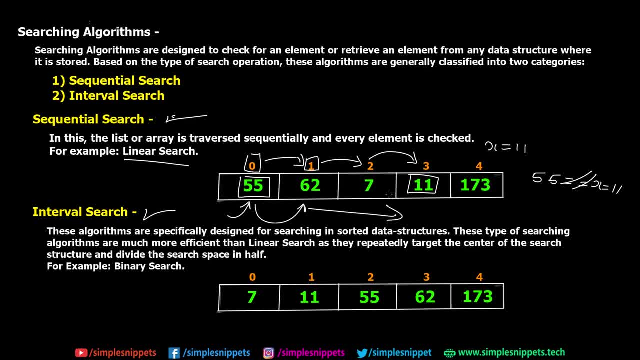 position to next and in that linear fashion. okay, so it does not check all the elements, But binary search algorithm is a type of interval search algorithm And these are the elements. these algorithms are specifically designed for searching in a sorted data structure. 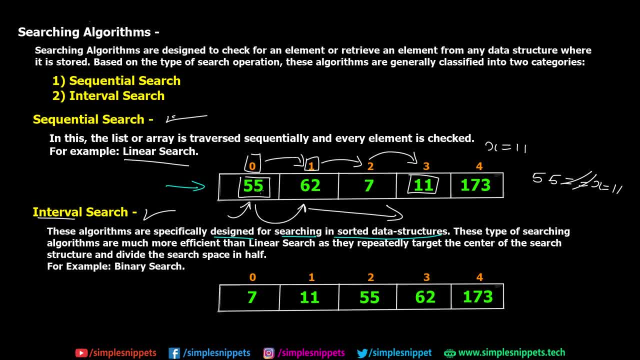 So, if you see, this array is not sorted in any order. it is not an ascending or descending order of the elements. But if you see, this is the same array, that is, it has all the same elements but it is sorted in ascending order, starting from the lower value seven. 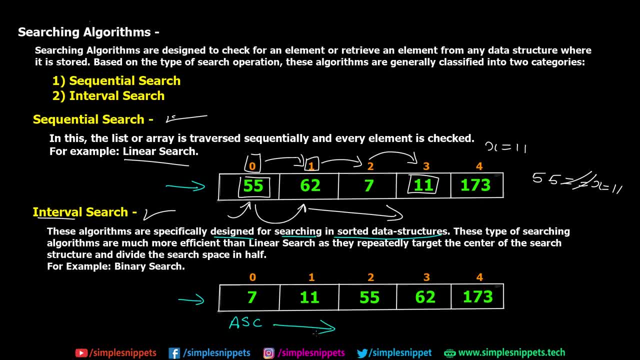 then 11,, then 55,, 62 and 173, in this order right. So binary search algorithm or interval search algorithms basically work on sorted data structures. only Now binary search falls under the category of interval search And these type of searching. 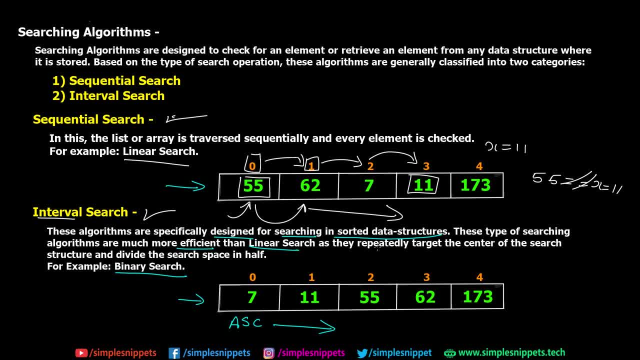 algorithms are much more efficient than linear search as they repeatedly target the center of the search structure and divide the search space in half. So of course we'll discuss in detail this line, But basically they are more efficient because they do not actually 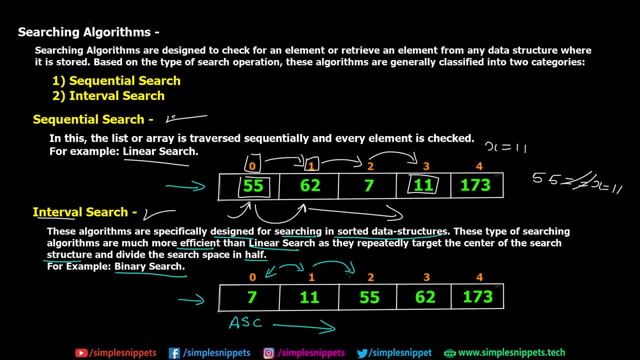 go one element to the next and to the next in a linear way. So they basically divide the structure or data structure into sub parts and only search through that which is essential. right, And of course we'll see the working now. So let's go to the working of binary search. 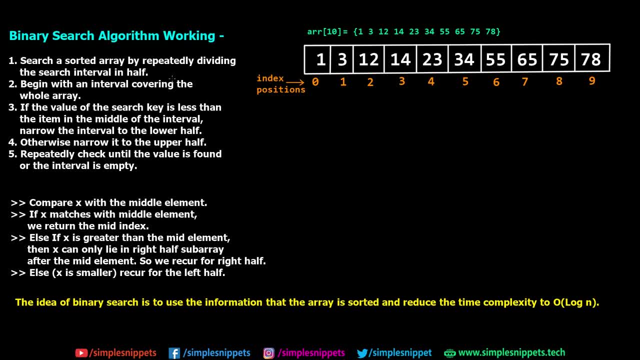 algorithm. Okay, so, as you can see, on the left hand side we have some description about the working of binary search algorithm And on the right hand side I have a diagram. So, let's say, we have a sorted array of size 10.. It has integer elements. you can see one. 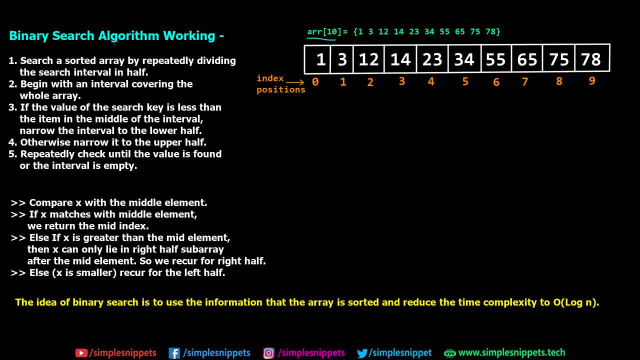 312, 1423, and so on. So let's see how the binary search algorithm would work on this array. Okay, so the working of binary search algorithm goes as follows: we have to search a sorted array or sorted list, basically by repeatedly dividing the search interval. 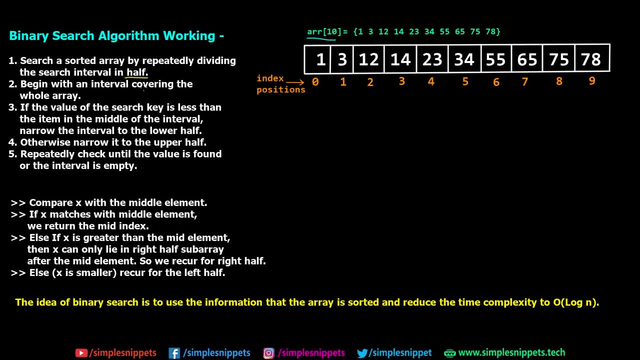 in half. Okay, remember this point. I have to begin with the interval covering the whole array. So the interval initially would be from zero to nine, right. So the left value of the entire interval would be zero and the rightmost value would be nine. Now, if the 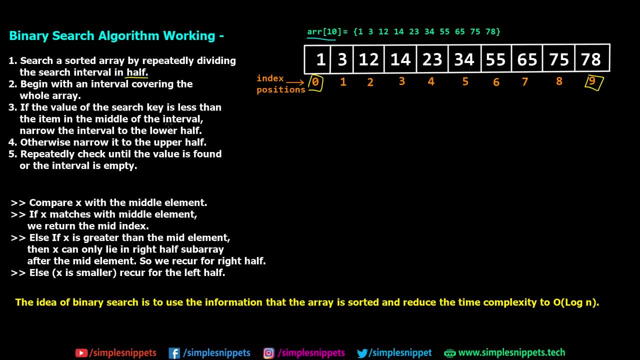 value of the search key is less than the item in the middle of the interval, narrow the interval to the lower half. otherwise narrow it to the upper half. If you didn't understand this, we'll again go to this point. But let's just complete the working. And we have to repeatedly check until the value 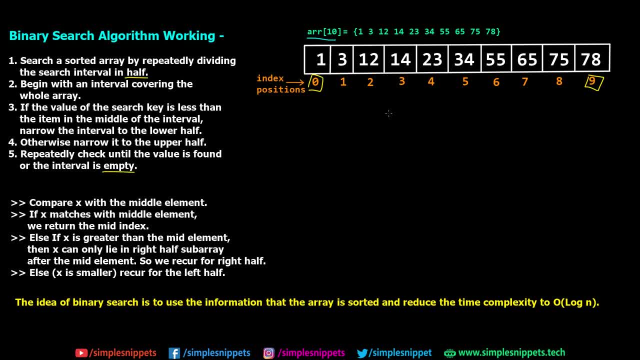 is found or the interval is empty. Okay, so let's assume you want to search for the value. x equals to 75, okay, So, on another way to put these, five steps are as follows: So you have to compare x with the middle element. So for the first time we have to calculate. 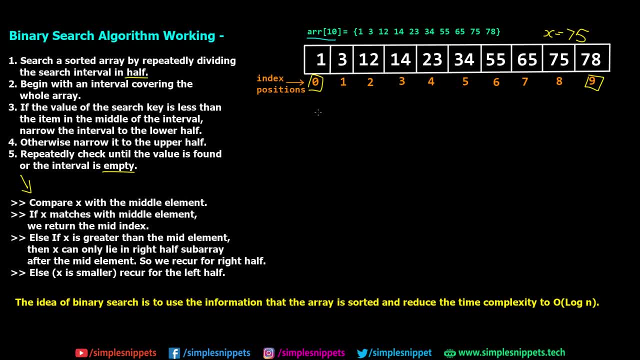 the middle element. So what we have to do is we have to take sum of left. so this is the left most value And this is the rightmost value, most value, right? so if you take a sum 0 plus 9 and divided by 2, so you'll get 4.5, but obviously 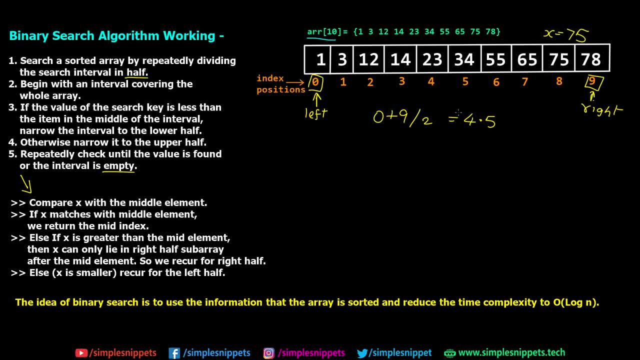 we don't have a 4.5 value index, we only have integers. we don't have fractional indexes. so we will just truncate this part, so we'll get 4. so right now, let's consider this as the midpoint. okay, so this is the mid. so we have to check x value with the middle element. so right now, this: 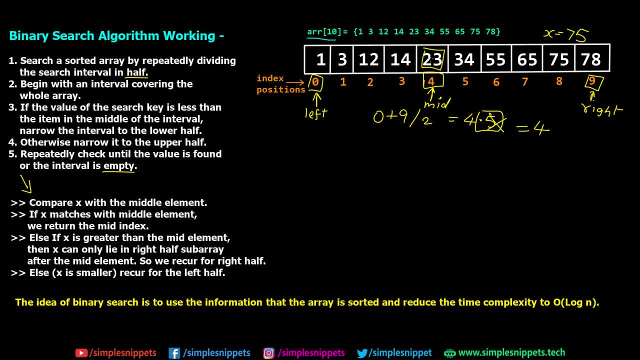 is the middle element. the element at this index 4 is 23, so i have to check with 23 and compare it with the value that you want to find out now. if x matches the middle element, we will return the mid index. so if there is a match, if 75 would have been over here, it would have matched with the 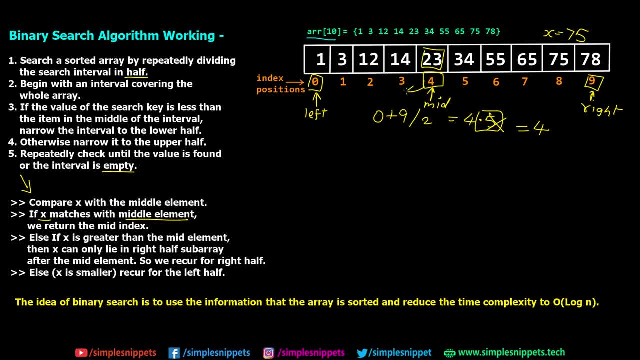 value that you want to search. right, then we would have simply returned this index position 4. that is, we found the value at index position 4. this is the output, right, but right now it is not matching right. so next step is else: if x is greater than the middle element. if x is greater than the middle element, which is currently. 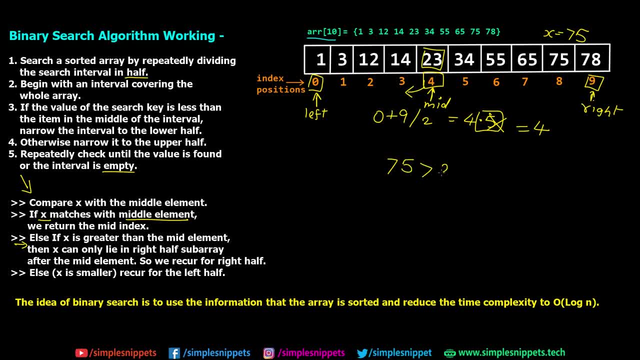 true right 75 is greater than the middle element 23, then x can only lie in the right half sub array. so essentially what we've done is we've divided the array into two parts, and this is the midpoint. so this is the first half, or you can also say left half. 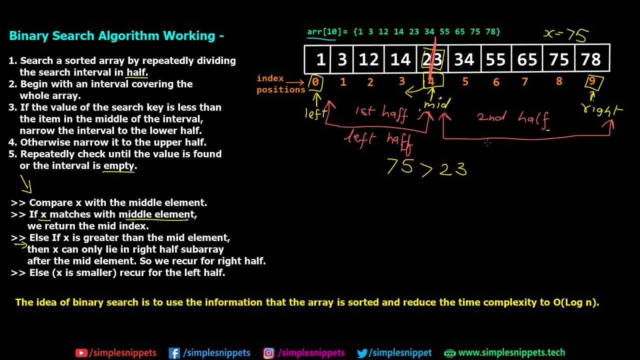 right, and this is basically the second half, or you can also say it as right half. okay, so now we know that 75 is greater than 23 and we know that the array is sorted, which means 75 will be obviously lying in this half, only right in the right. 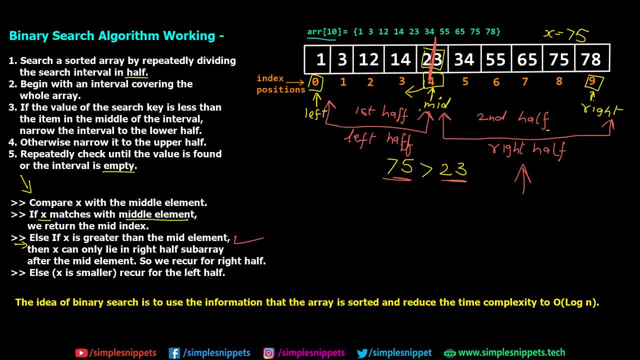 it. so that is why this else if condition will be true. so now we will only search through the second half. we don't have to search through index position zero, we don't have to search through index position one or two or three, because you already know that since 75 is greater than 23, our value 75 if it is an 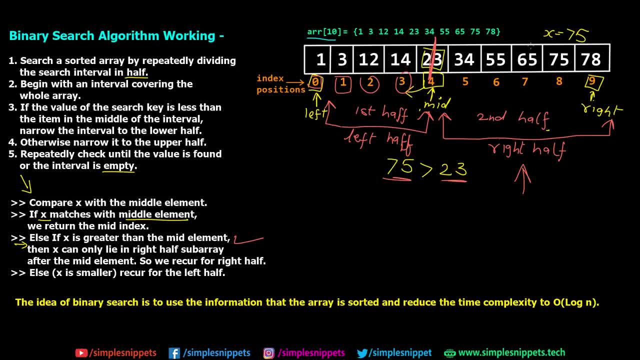 ness, position zero. you don't have to search through index position one or two or three, because we already know that since 25 is greater than 23, our value 75, if it is existing in the array, it will always exist in the second half because it is a sorted array and hence we require sorted array and 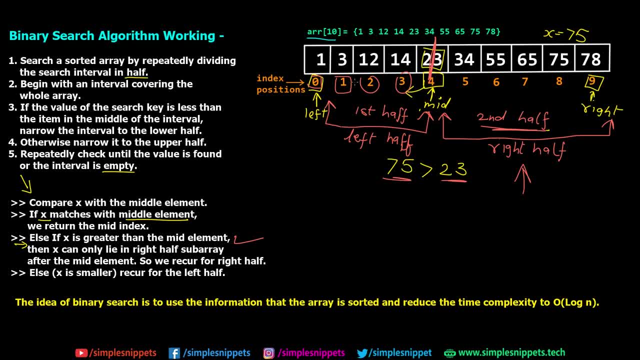 binary search algorithm only works on sorted array right. so now for the next iteration. because we did not find the value at the midpoint, we will further carry out all the operations on this second subarray only. so again, we will calculate the mid. so for now, this is the new. 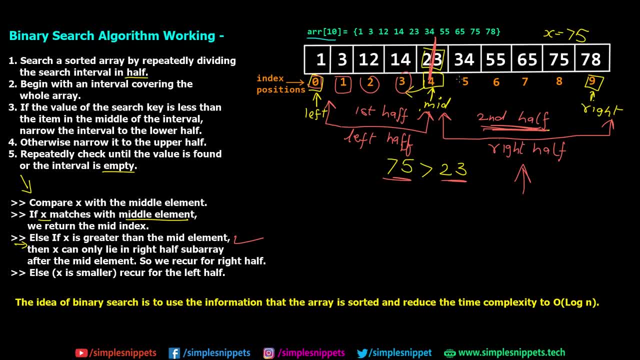 left, right. so we will say: left is equal to mid plus one, so the new left will be this one and the right will be as it is okay. so let me just erase this all out. so, as you can see, now we are only searching in the second half of this entire array, because we've concluded. 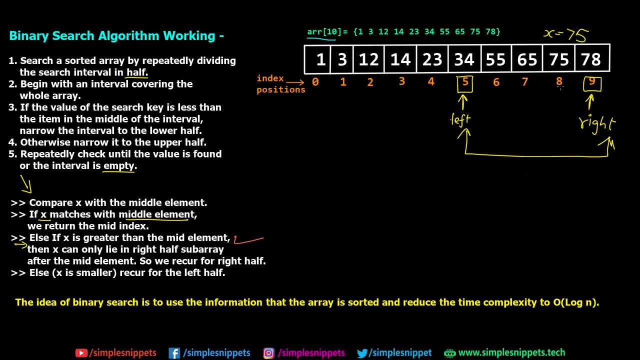 that, since 23 was less than 75, we only have to search the right hand side. so now again, we will calculate the midpoint. how do you calculate the midpoint? you take a total of five plus nine. you just divide it by two, it would be 14.. 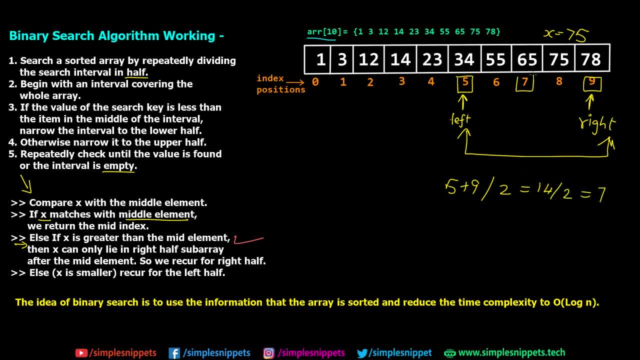 by two, so you'll get the midpoint of seven. so now, this is the midpoint, so this is a new midpoint. okay, so this is the second iteration and we got a new midpoint. so now, again, we have to check the value at this midpoint, and we know that 65 is less than 75, right, or you? 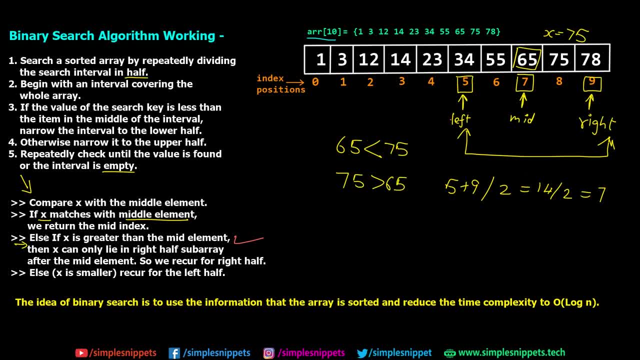 can also say: 75 is greater than 65. so again, this statement will be again true. that is, x is greater than the value that we are getting at the midpoint. so now we will again know that we have to check the value at this midpoint. so now we will again know that we have to. 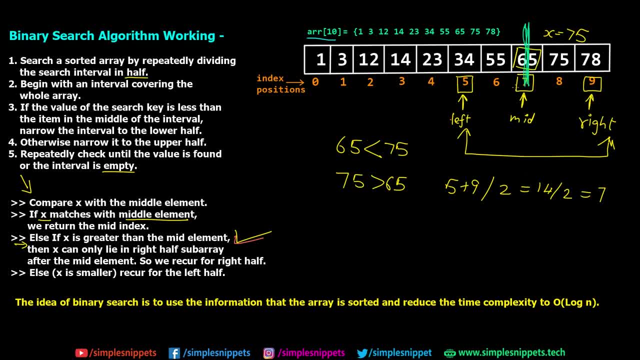 divide this small array into further more two parts. so this is going to be the first part and this is going to be the second part. right, first and second. and since 65 is less than 75, we know that our value is going to be lying in the second half only. so now we 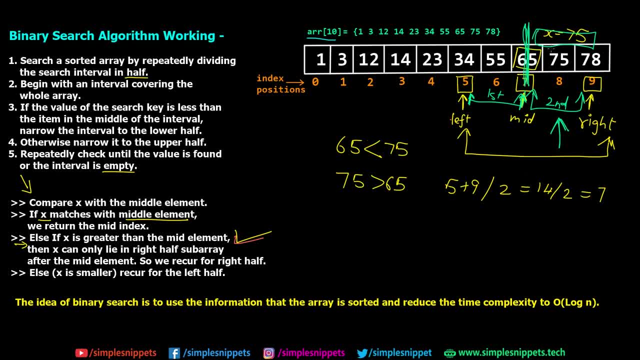 are only interested in these three values or these three index positions. so, again, we will search and this process will keep on repeating till we actually find out the midpoint. okay, so this was just the theory and work. Thank you for watching. And one last thing that I wanted to talk about is the idea of binary search, is to use the 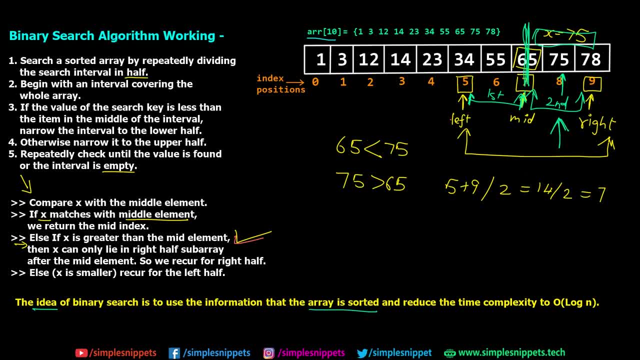 information that the array is sorted, because obviously, as we see, binary search algorithm will only work on sorted arrays and the time complexity is reduced to o log n. now we've not discussed about time and space complexity and those asymptotic notations, because I first want you guys to understand these different algorithms. so after we complete the searching, 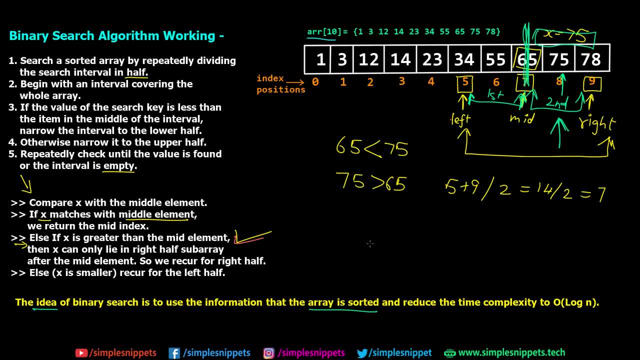 and sorting algorithms. we will take a separate look at the asymptotic notations and those different time and space complexity concepts. so if you're watching this video in the future, those videos might already be up in the DSA playlist, so do check it out, if not definitely. 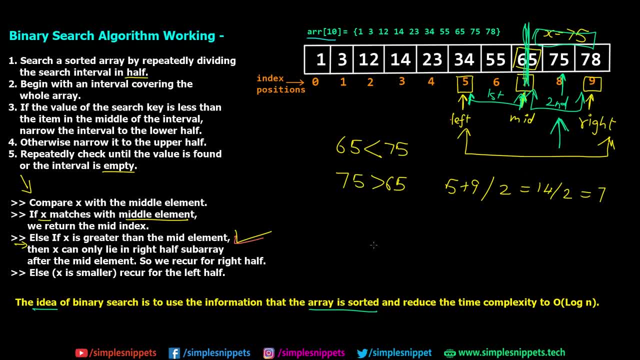 subscribe and turn on the notifications, because those videos will be uploaded soon. okay, so this was just the theory on binary search algorithm and I hope you've got a rough idea about how it works. now let's take a look at the algorithmic statements and how the pseudocode 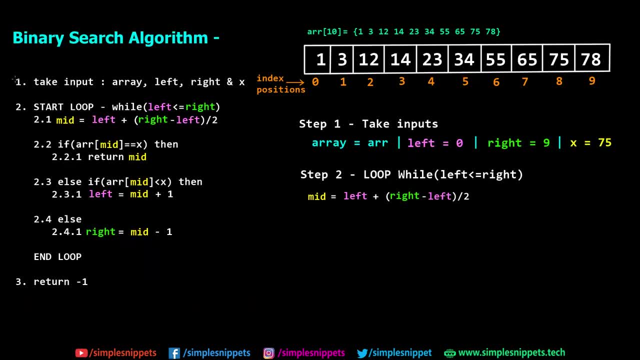 would look like: okay, so, as you can see on the screen, this is the binary search algorithm in the form of pseudocode. Step number one, Step number two: inside step number two, we have multiple steps, which is a basically a loop, and then we have step number three. okay, so the first step states that we have to take. 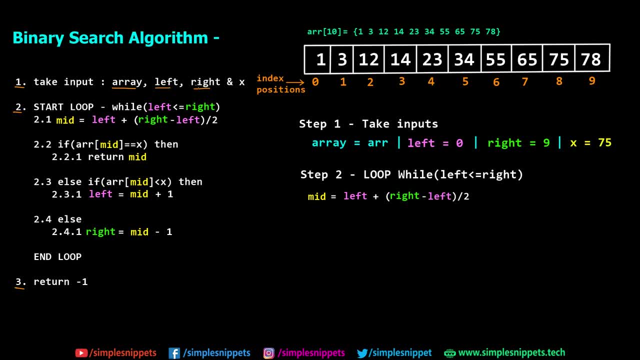 input. we have to take the array. we have to take the left and right intervals and the x value that we want to find out. so, step number one: take inputs written over. here we take the array arr. so this is our array. initially the left value would be zero, right? so this? 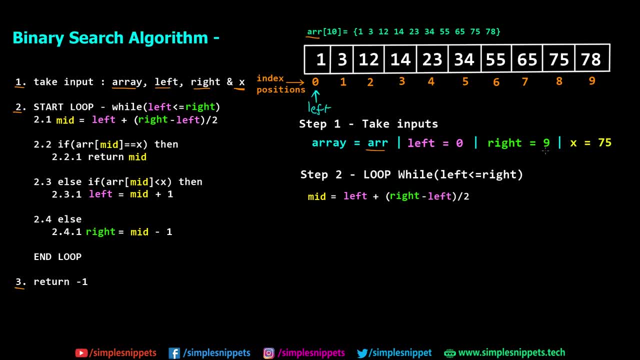 is left. let me use another marker. and the right value is nine, which is the last index position, And let's assume you want to search for the value of 75, which is somewhere over here. right, this is that value. So we take the input now. step number two is start the loop. and now the condition is why. 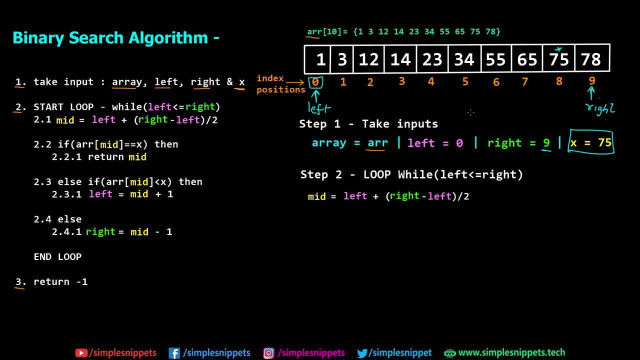 left is less than right, while this left index is less than the right index. it means that we have some interval, some values in between. so we have to keep on iterating this loop till left is less than equal to right right. we have to divide this array into halves every. 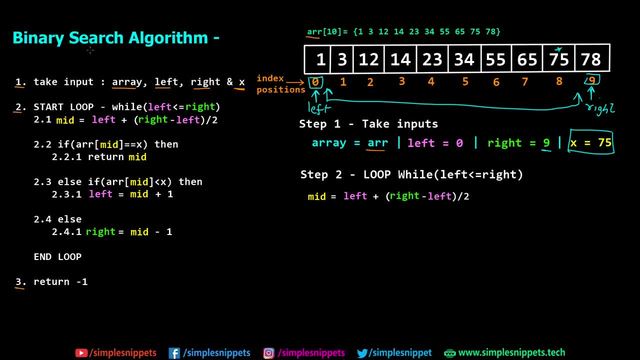 time, Until until and unless you find a match right. This is how the binary search algorithm works, So this is going to be our condition. So, for starters, obviously left is going to be less than right. left is zero and right is nine right now, So this condition would be true. 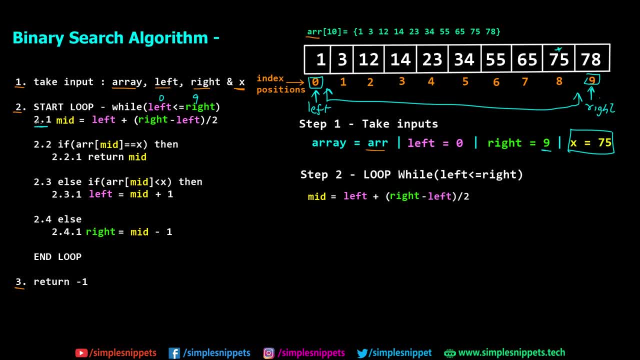 So we will go inside this loop while loop and we will execute step 2.1.. Now, at step 2.1, we are calculating the mid value which is given by left plus right minus left by two. So let's calculate that left is zero plus right minus left, which is nine minus. 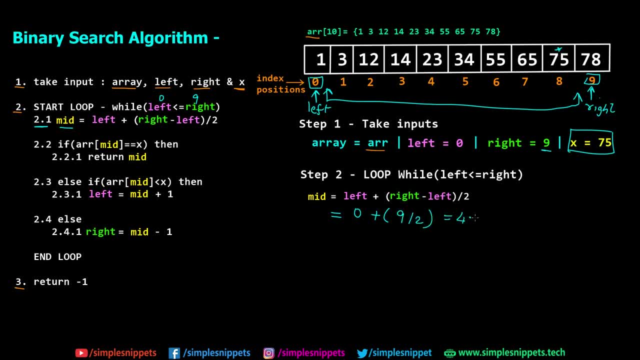 zero, So nine by two, so this is going to give you 4.5, which is basically four, because we don't have 4.5 index and we are playing with integers. So when you actually convert this into a program, this would be an integer value, int. mid. Okay, So it will only store. 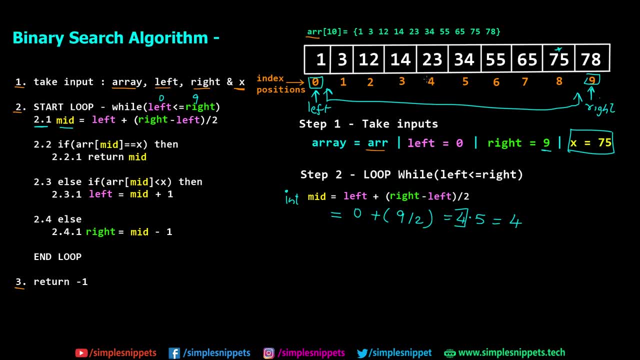 the integer part and not the floating part. So now we've calculated the mid value. This is the mid value. So we move on from step number 2.1 to step number 2.2. So we are still inside the loop. 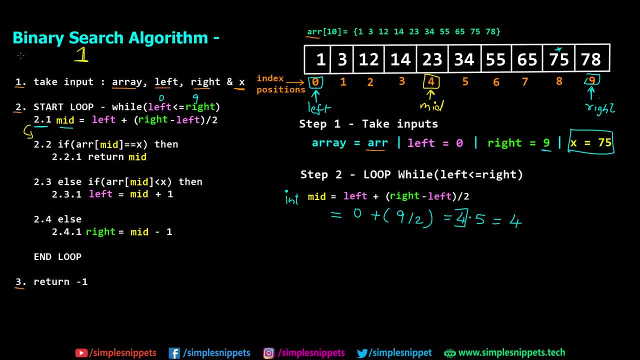 This is basically our very first iteration. I'll write the iteration number over here. So in step number 2.2 we check if ARR of mid equal equal to X. So whatever the mid value we found out, index position, we check the value at that position, which is 23.. We try. 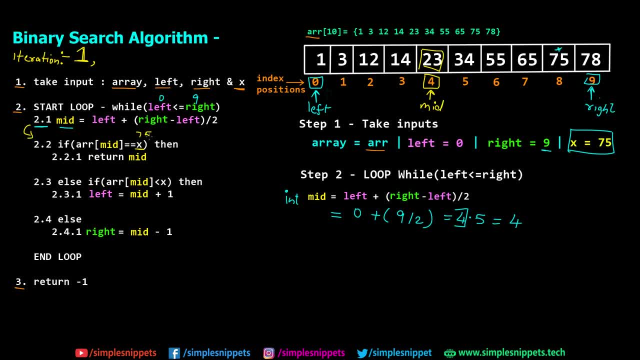 to match it with our X value. X value is 75 and mid value is 23.. So obviously this is not going to be a match. So this if condition will not be executed at 2.2. So we will move on from 2.2 to 2.3.. Here we are checking. else, if ARR of mid is less than X, ARR of mid is: 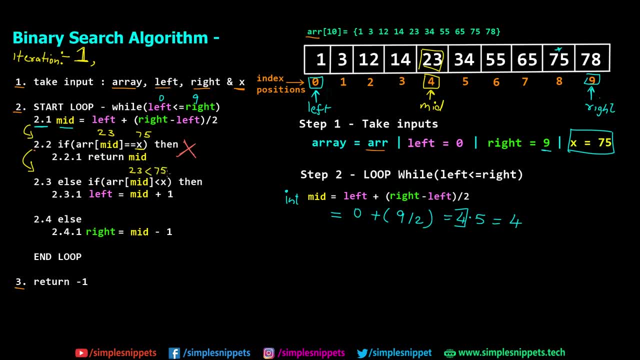 23.. 23 is definitely less than 75. So this condition is true. So now we will execute this 2.3.1, which is inside 2.3.. And here we are saying: left is equal to mid plus one. 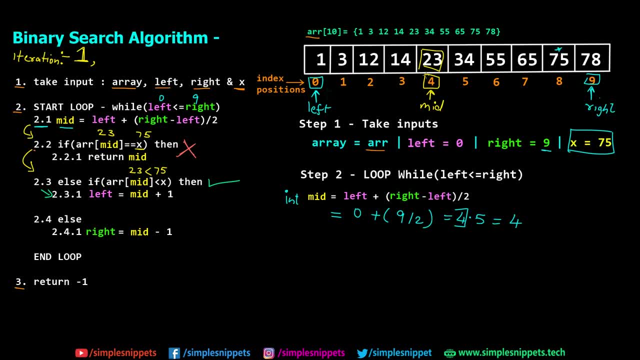 Left was zero initially. Mid was 0. Because this value four, So four plus one will give us equal to five. Okay, So now we just changed this left to value five, So let's make that change over here. So the new left. 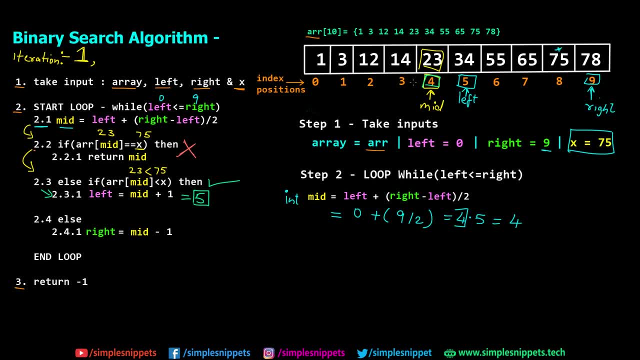 value is this index position five. Now, obviously, the reason why we did this is we know that 23 is less than 75. So we know that the value 75 that we want to find out is obviously going to be to the Second half of the array. So this is the second half And this is the first half We divide. 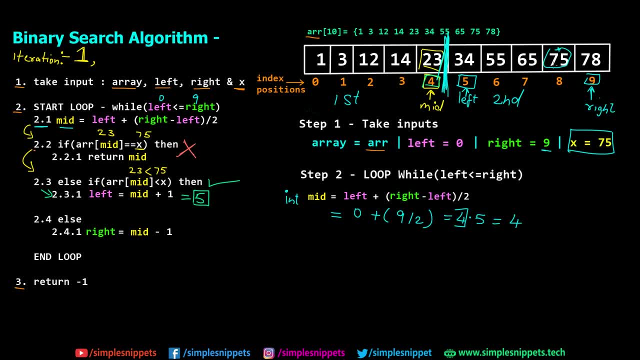 it at this midpoint Right. So since 23 is less than 75, the 75 value is always going to be lying towards the right. That is the second half, because this is a sorted array. So that's why now we will only check between these two positions. So the interval has become: 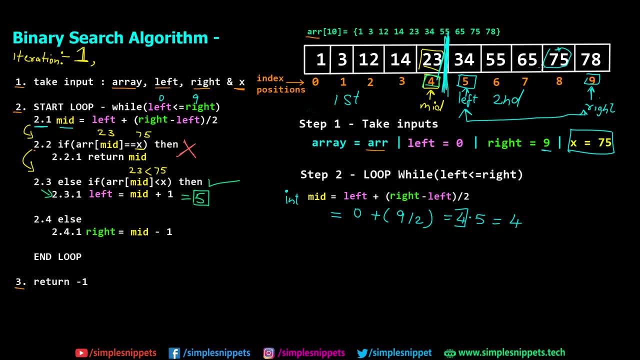 smaller now, okay, From zero. now the interval is between five and nine And of course after else, if we will come to the end, we will not execute step number 2.4, because this is a else part. so either if part else, if part or 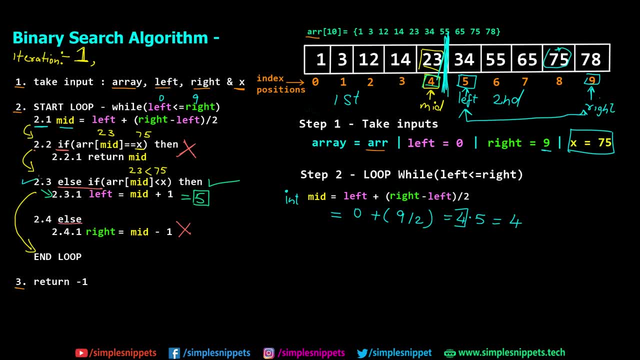 else part will be executed and since we just executed 2.3, we will not execute 2.4. we will come at the end of the loop and now we will go at the start of the loop again. at the start of the loop we will check while left is less than right. we just change the value of left and the new value 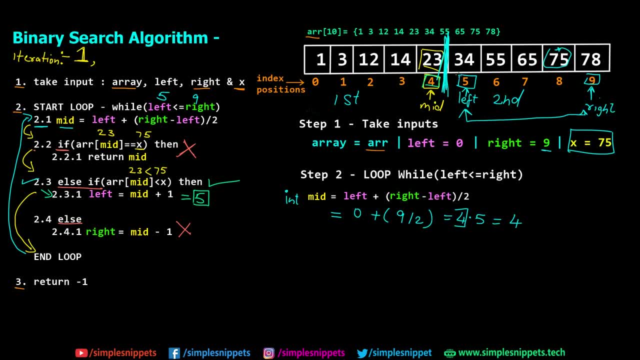 of left is 5 right. we just got over here new value of left, which is 5. so 5 is still less than 9 right, which means we still have some interval to cover. so again, the condition will be true. we will start with our second iteration. so let me just clear out the screen. so now we will again. 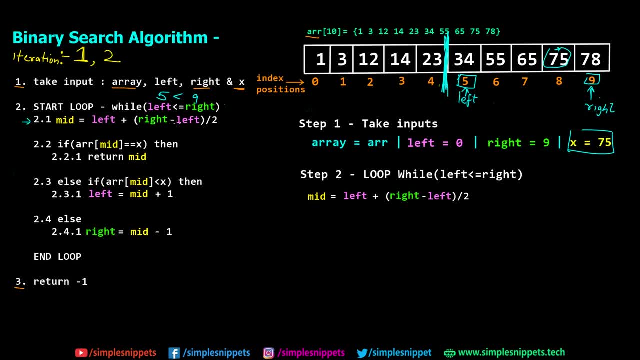 calculate the new midpoint. so midpoint is equal to left plus right, minus left by 2. the new value of left is 5. you can see from the diagram over here: plus 9 minus 5 is 4 by 2, which will give us 7 right. so the new midpoint that we find out is 7. coming to step. 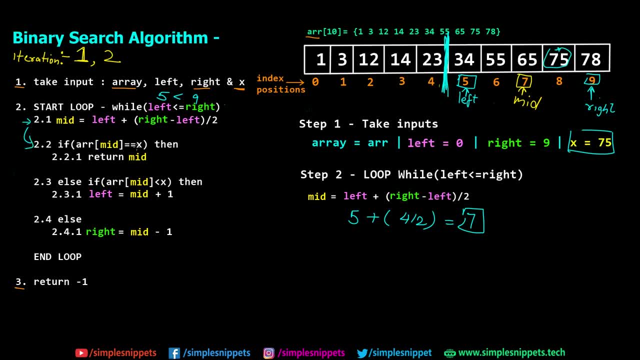 number 2.2. we again check: if arr of mid equal, equal to x, arr of mid, which is arr of 7, it is 65. is it equal to 75? no right, it's not. so this statement becomes false. so this if condition will never be executed at this iteration, we will come to step number 2.3. now we compare: if arr of 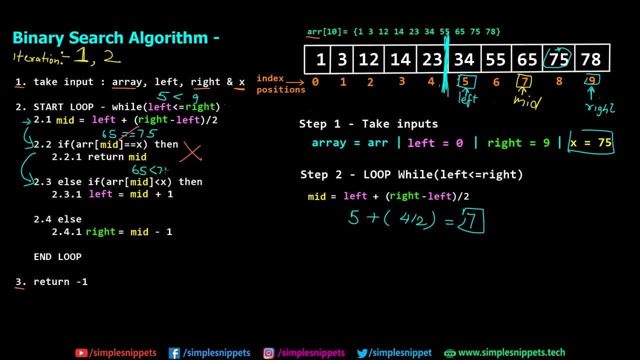 mid is equal to 7, right. so this, if condition will never be executed at this iteration we will come. that is, 65 is less than 75, this is true, right. so again coming to step number 2.3.1, we again reduce the interval. we say left is equal to mid plus 1. we just calculated mid as 7. 7 plus 1 will 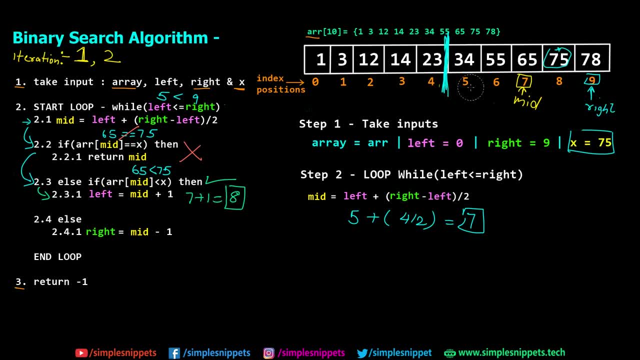 be 8, so let's change that, so our new left would be 8. okay, so obviously, since 65 is less than 75 and this is the midpoint, we know that our value has to be somewhere in these index positions and not in these index positions, right, so we don't have to search for them in this this? 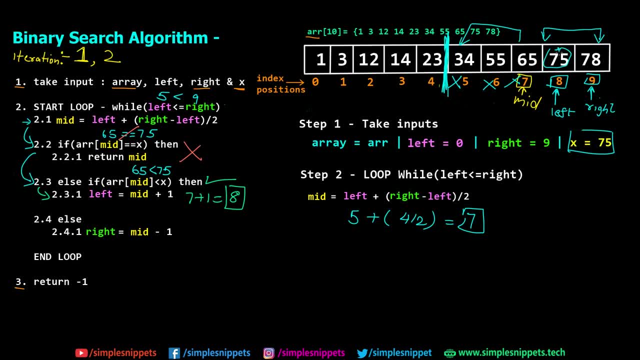 and this part. we know that 65 is less than the value that we want to find out, so it has to be there in the last two values only. so that's why we again divide this subarray into more smaller arrays, and we are only interested in the second part of this subarray, right. so from step number. 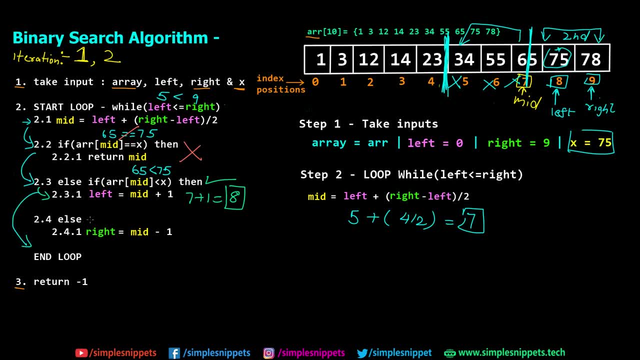 2.3.1, we will again come to the end. we will not execute the else part, because we just executed the else if part. so from here we will again go to the start of the loop. and now we will again check. while left is less than equal to right, the new value of left is 8. so you can see, 8 is still less than 9. 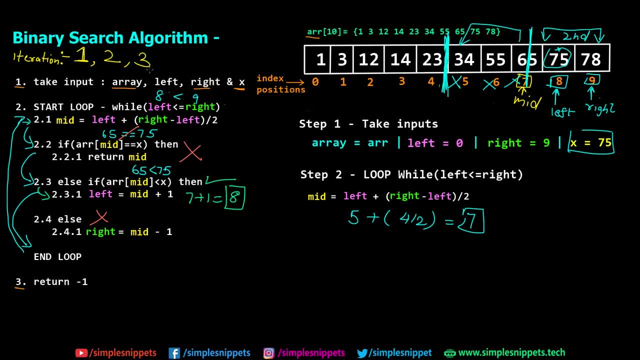 so again, we will now start with the third iteration. let me write it over here, let me erase this out. okay. so, coming inside, we again calculate the midpoint. midpoint is given by left, which is 8- you can see index position- 8 plus right, minus left, which is 9 minus 8 by 2. 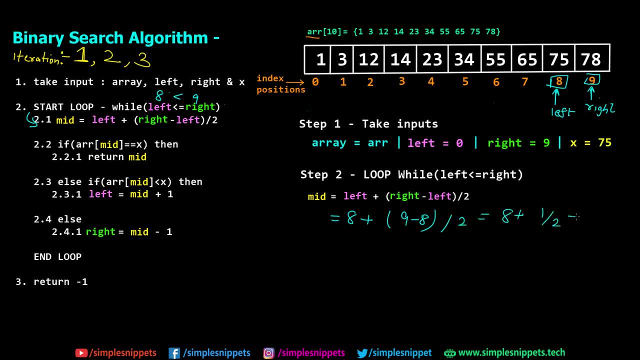 so this would be 8 plus 1 by 2, which would give us 8.5, but ultimately we will truncate the floating point, so ultimately we will get the midpoint of 8. okay, so now this is also our midpoint. coming to step number 2.2, we will check if arr of mid, which is arr of 8, that is, 75, is equal to our x value. 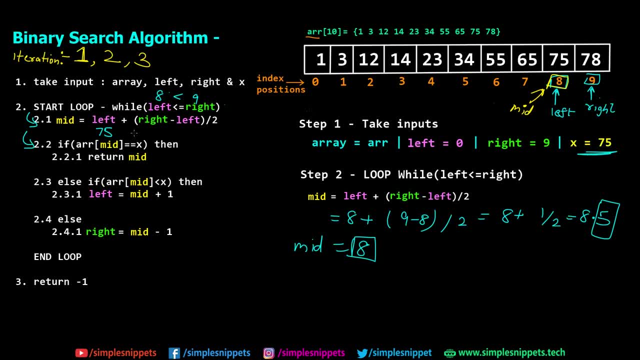 now our x value is also 75, right, so we want to search for that, only so we will get a match over here. so now we are going to search for that only so we will get a match over here. so now we are. now this statement becomes true, so we will execute 2.2.1 in the third iteration. i mean we will just 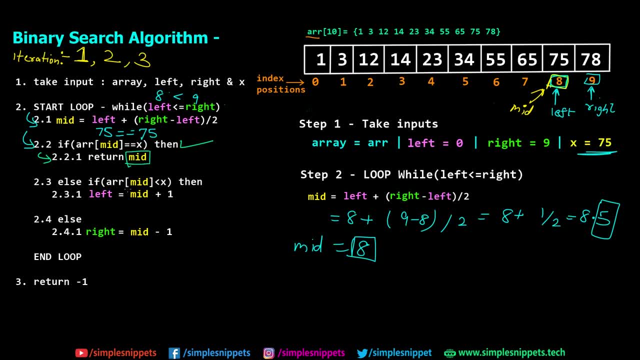 return this index position mid and this is where the algorithm will stop. so you can see that in three iterations we got our result and we got our match at this index position. now, if you see, if you would have started with linear search algorithm, what would have happened is in the loop we would. 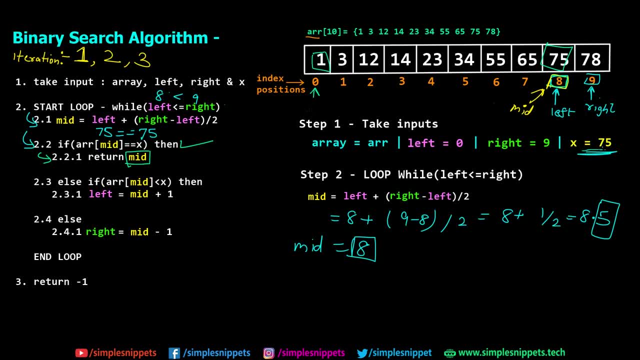 have started from this position, we would have matched 75 with the index value of 0, which is 1. then we did not get a match. we would have jumped to index position 1, again, no match. so again jumping to the next- no match. jumping to the next- no match, and so on and so forth. so you can see the number of hops that we 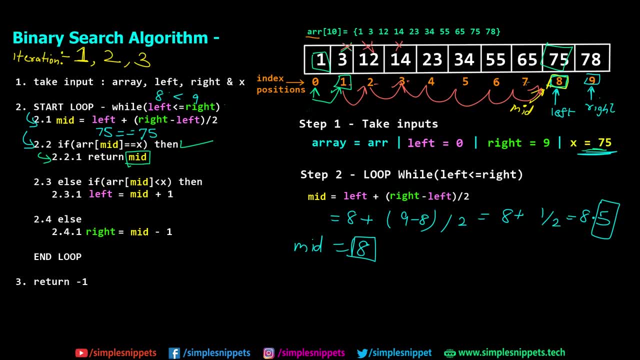 would have required is 1, 2, 3, 4, 5, 6, 7, 8 and at the ninth iteration we would have found our match. but using binary search we only required three iterations of this while loop, but if we would have used the linear search in the for loop we would have required nine iterations. 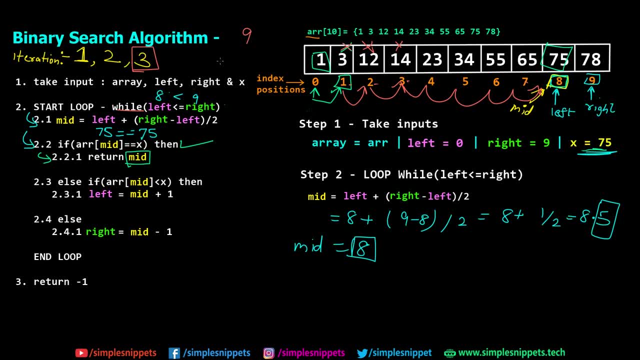 so you can see, binary search was much more faster, provided that we have a sorted array right. so this is the power of binary search algorithm, and i hope you understood the algorithm as well and the working with the diagram. now in case, if the search value that we wanted to search would have been, 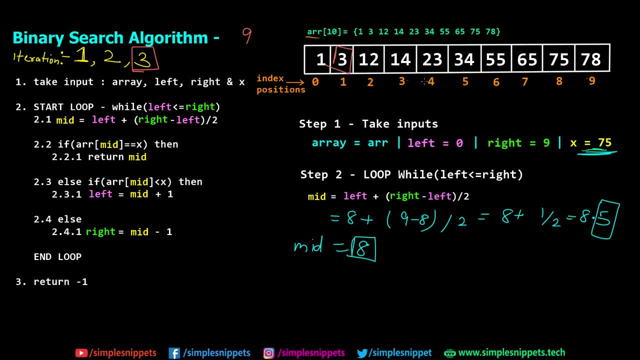 somewhere over here. then first we would have calculated the mid. so let's say again: we are at the first iteration only. okay, so this is iteration number one. instead of x equals to 75, we want x equals to 3, so we would have calculated the mid initially. this would be the left and this would 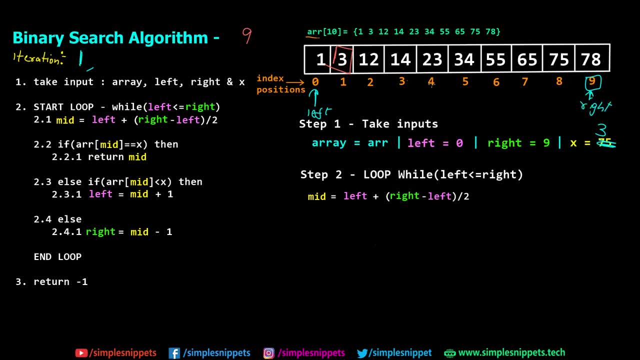 be the right. for the first time we calculated the mid as 4 right for the first iteration by using this formula: mid is equal to right minus left by 2 plus left, so that would give us 4. so now we would have checked over here. if arr of mid equal equal to x, so is 3 equal equal to x, that is, is 23 equal. 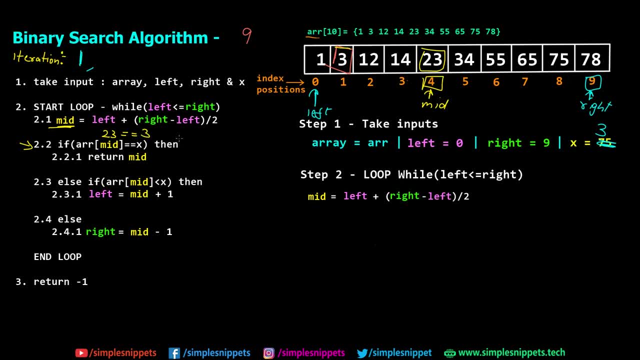 to the value that you want to find out, which is 3, not true, right then we would have come to 2.3. we would have checked if arr of mid is less than x. so arr of mid is 23 over here is 23 less than the. 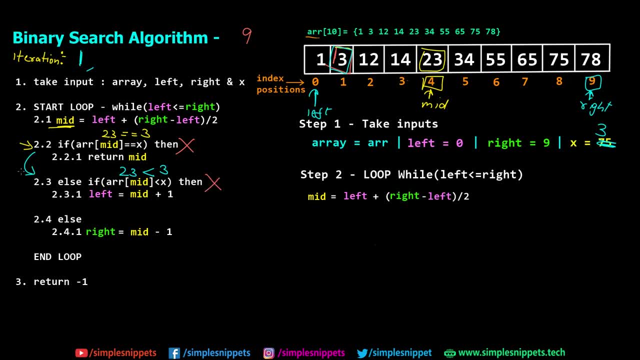 value that we want to find out, which is 3- again false. so in this case, step number 2.3 will not be executed, but step number 2.4 would have been executed. and here what we are doing is, since we know that 23 is greater than the value of x, which is 23, we would have found out that the value of x is 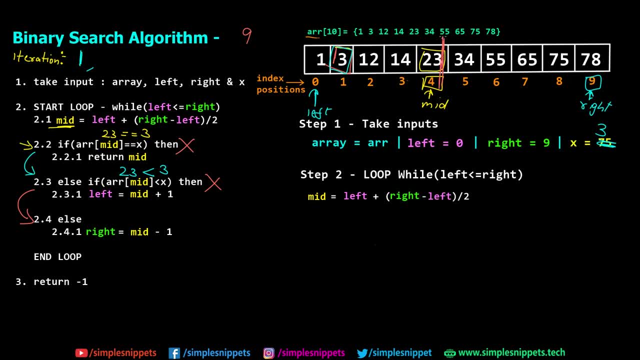 that we want to find out. If we divide this area at this midpoint. we know that we are having two halves, So this is the first half And this is the second half of the main array, But since 23 is greater than three, we know that our value will be lying in the first. 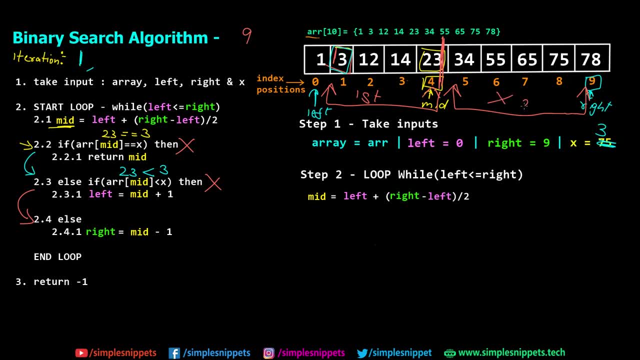 half now right, And not in the second half, because this is a sorted array. So now, instead of changing the left value- which was happening at step number 2.3, here we change the right value, that is the right interval, and we say: right is equal to mid minus one, So mid. 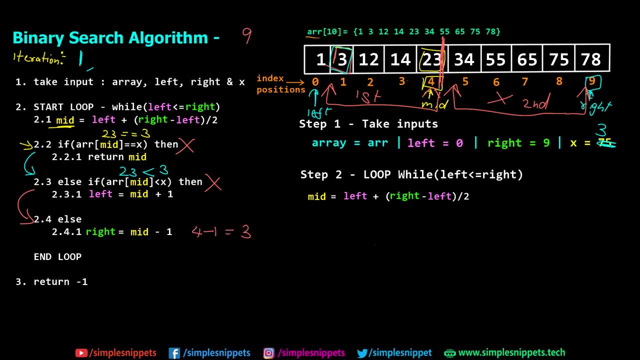 is four, So four minus one would be three. So now this right interval would have changed And now it would point to this position. So now we are only interested in the first half and not the second half. Okay, So this is that else condition, And of course then we 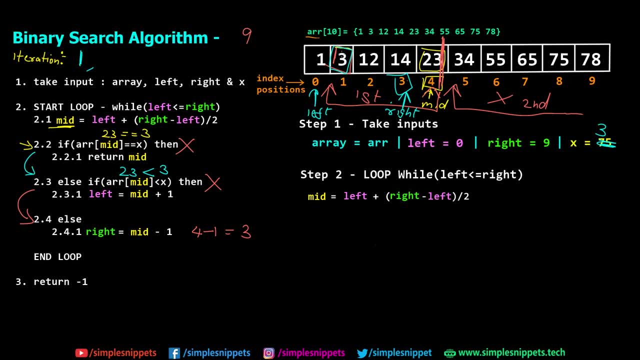 would go with multiple iterations. this interval will become shorter and shorter until and unless you find our answer. And one last use case was: let's assume that we enter a number: X equals to 115. Now, 115 is not there in the area, only right. So in that case, this interval. 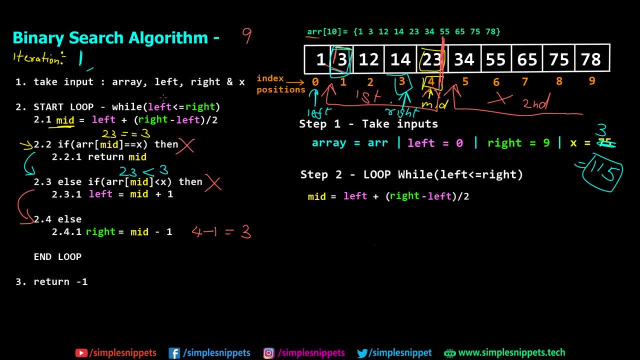 will actually come to an end wherein the while loop condition will become false and left value will become greater than right. In that case, this loop will exit out and ultimately we will return minus one at step number three. So this step number three will only be executed. 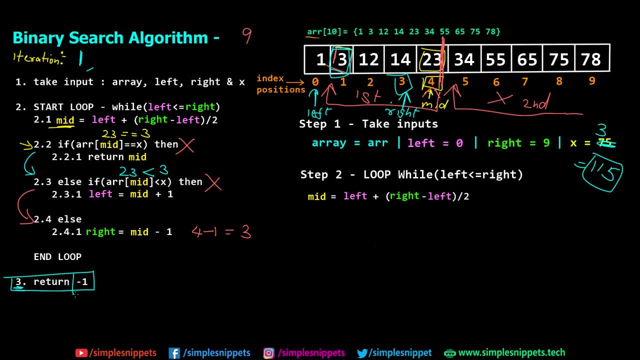 when we do not find a match in the array And when we return minus one in the program, we can determine that Since we have returned a minus one and minus one index position does not exist, right, We don't have minus one index positions. So in the if else we can check if the value returned from the binary. 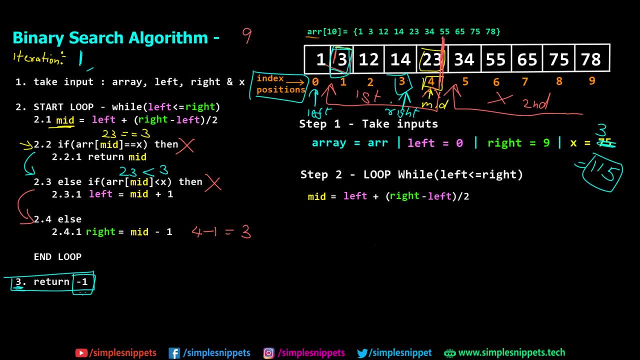 search algorithm function is minus one. if it is minus one, then we did not find a match, And other than minus one, if we get an actual value, then it would definitely be the index position of the value which is placed in the array. Okay, 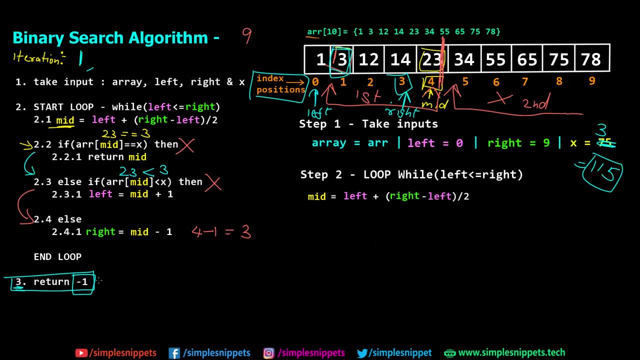 So this is why we've said return minus one over here, to indicate that we did not find anything matching in the entire array. So yeah, this was the complete working of binary search algorithm. I hope you've got a very clear idea about what exactly is binary search. 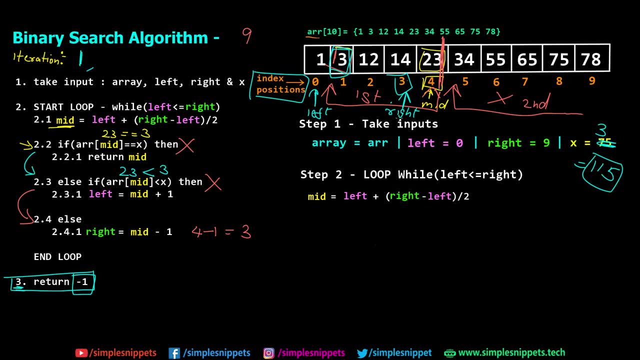 how it works, the entire algorithm as well as the diagrammatic representation. In the next video, we will implement this binary search algorithm using C++ programming and things will be more clear on the implementation side. So that's it for this video, guys. If 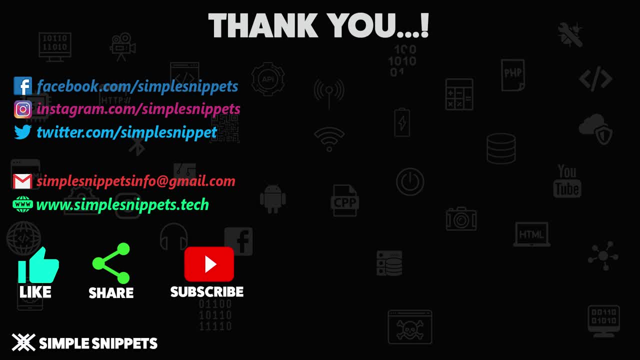 you like this video, please give it a thumbs up. Let me know in the comments how this video was. If you have any queries, you can put them in the comments And I will see you in the next video. Bye. If you haven't yet subscribed, please make sure to subscribe so that you get notified. 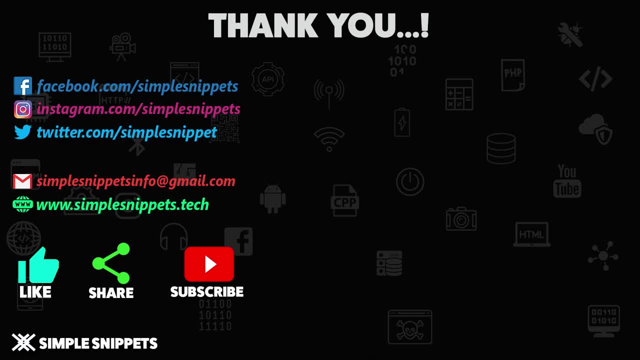 whenever I upload the next video, And I'll see you guys in the next video. Peace.